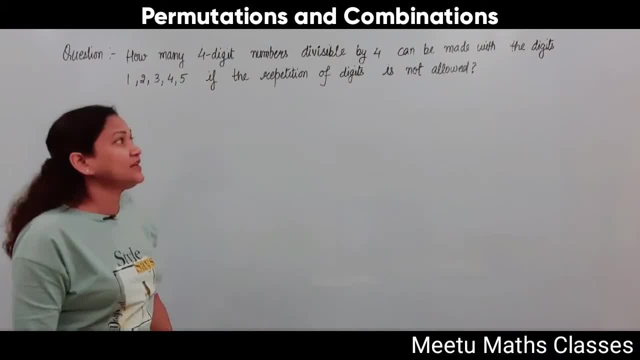 of digits is not allowed. all the four digits must be distinct. So let us try to find out the number of such numbers. So we are supposed to find four digit numbers and they must be divisible by four. And what does the four digit divisibility rule say If the last two numbers are divisible? 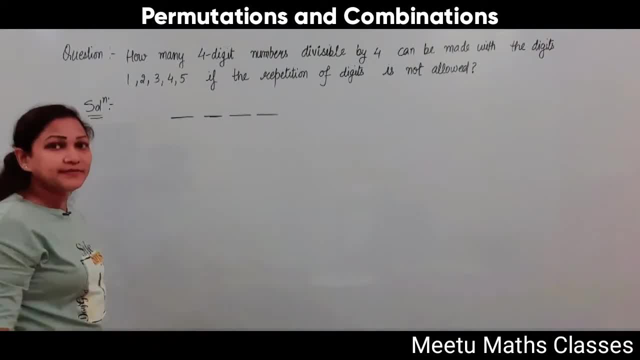 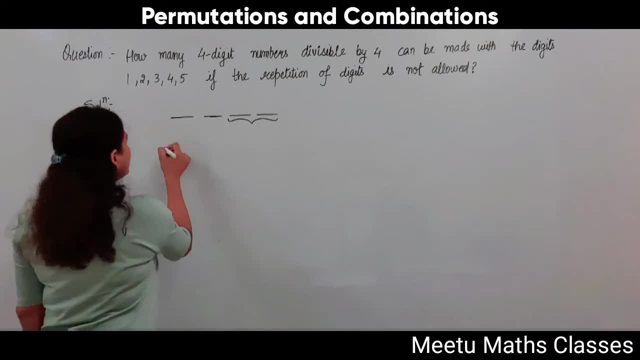 by four, then the whole number is divisible by four. So let us consider about the last two digits. What can be the last two digits? The last two digits can be your first number which is divisible by four, That is 0, 4.. Two digit number. So 0, 4 is not possible. Then 0, 8 is not possible, Then 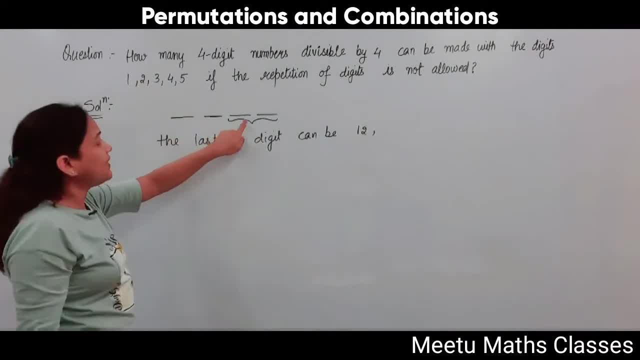 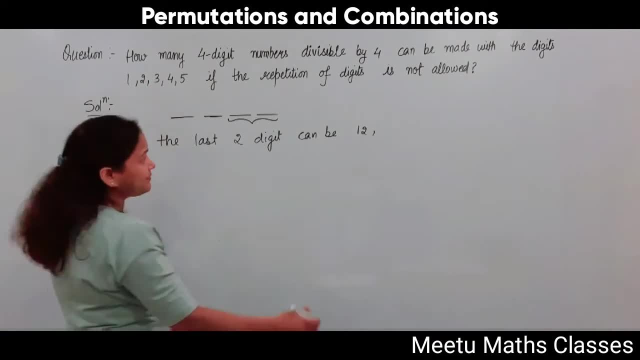 1, 2.. Yes, 1, 2 can be the last two digits. Then 1, 6 not possible. 2, 0 not possible, Then 2, 4 is possible, Then 2, 8 is not possible, Then 3, 2.. 3, 2 is possible, Then 3, 6 is not possible. 4,. 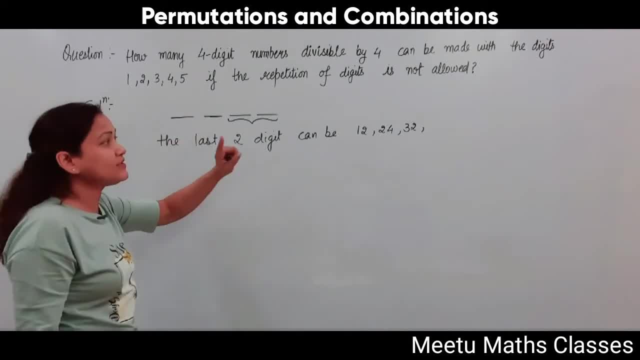 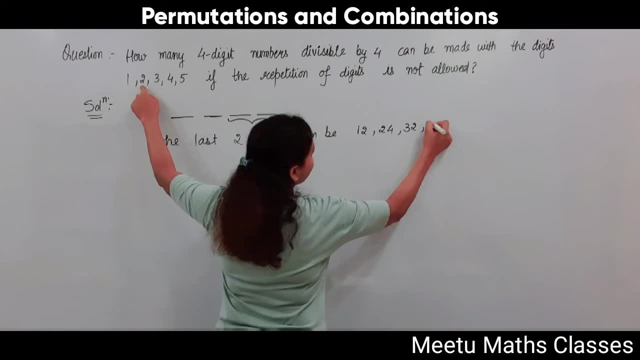 0 is not possible, Then 4, 4 is not possible because repetition is not allowed, Then 4, 8 is not possible, Then 5, 2 is possible, Then after that 5, 6.. So these can be the number of ways. 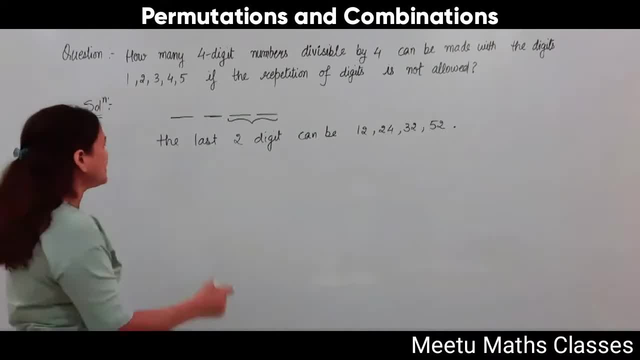 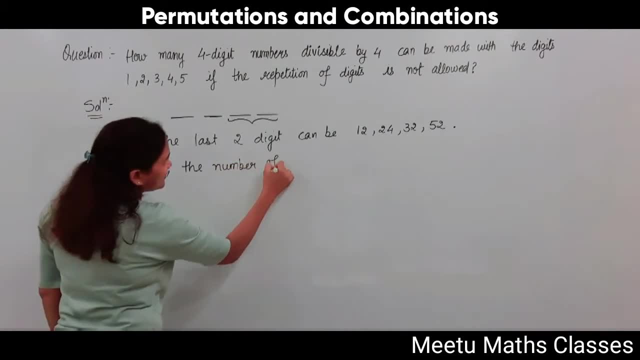 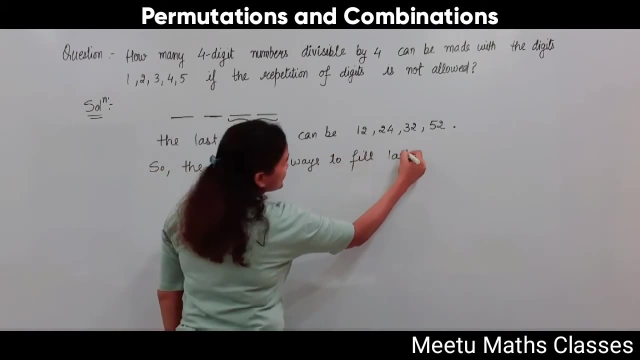 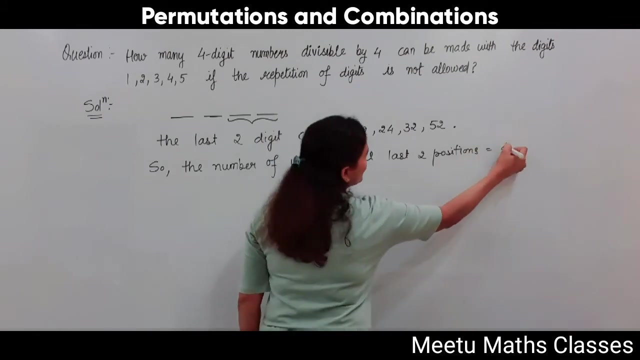 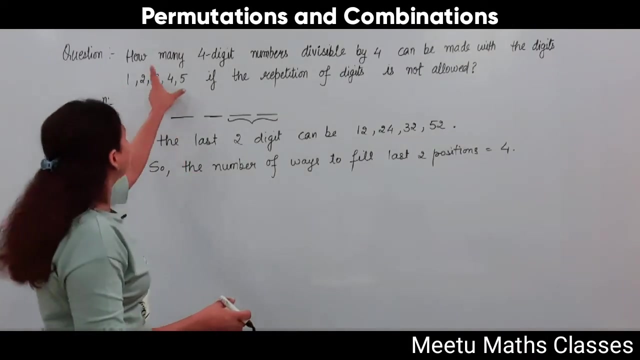 in which we can fill the last two positions. So the number of ways ways to fill last two positions will be 4.. So there are 4 ways to fill the last two positions. Aur D Cathedral. out of these five distinct numbers, two have already placed in at the last two places.